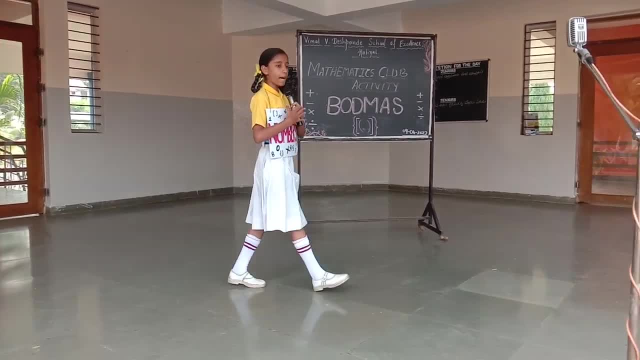 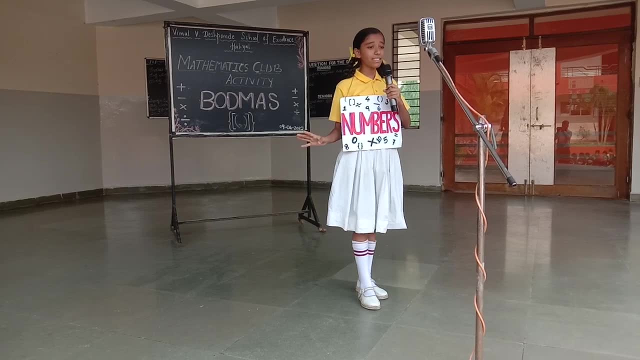 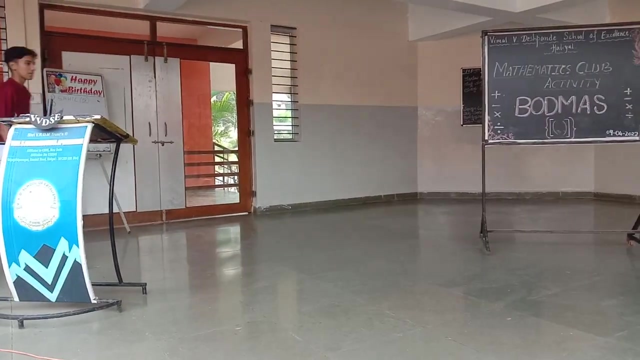 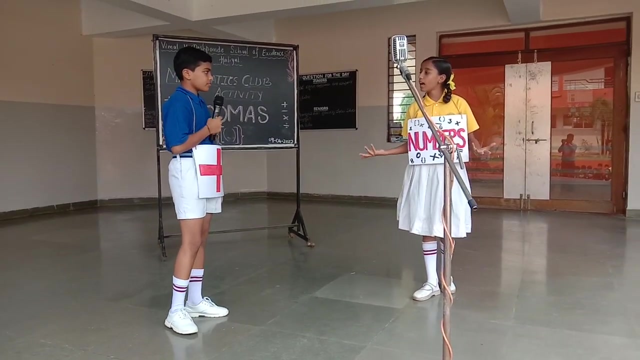 Problems, problems, problems. My life is full of problems, Dull and boring, Counting, counting, counting, Always counting. I am so alone with problems. Yo yo, yo, yo yo. Hey, who are you? Who allowed you to come in? 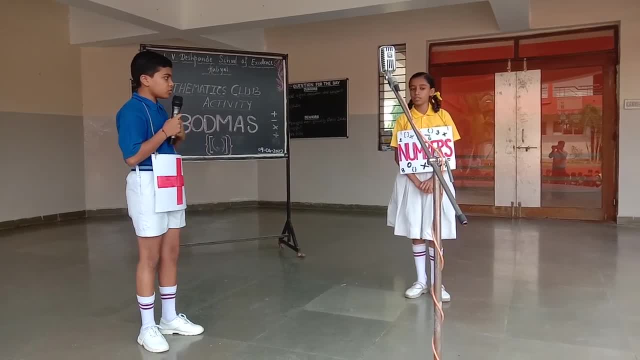 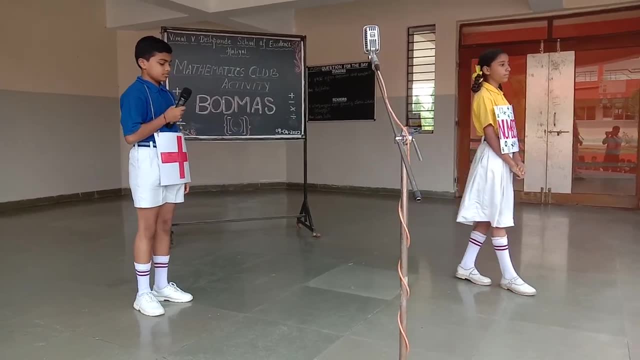 I will introduce myself. I am Adishan and I will prove that I am very intelligent, I am very useful to you, I can increase your value, So please don't try to avoid me. But how can you do this? 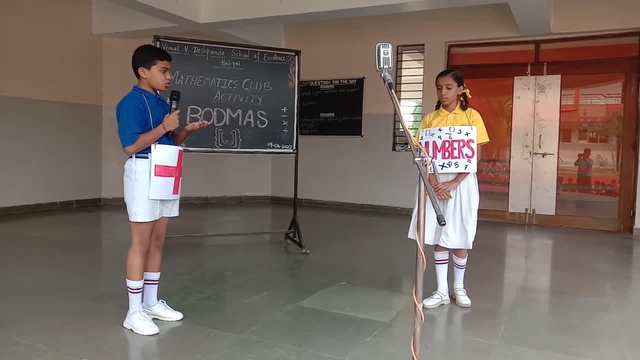 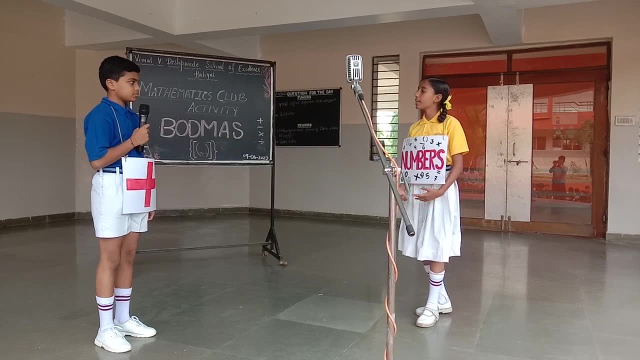 First take the number 3 and 2. If you add these both numbers, the answer is 5.. Oh wow, With Adishan we can make so many new numbers. I am so happy. But can you tell me how can I decrease my value? 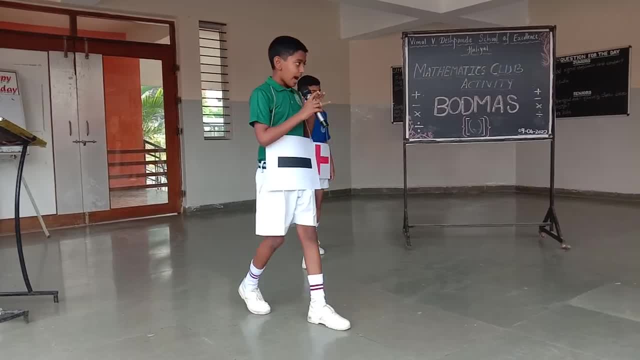 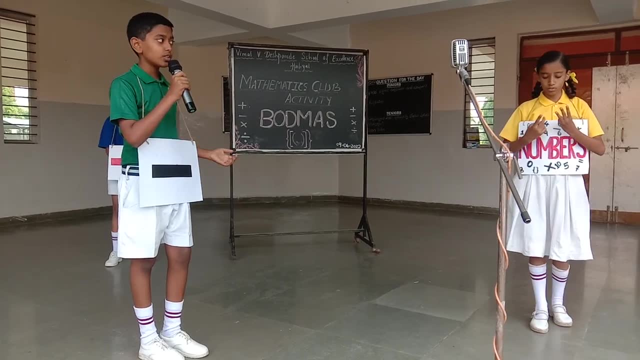 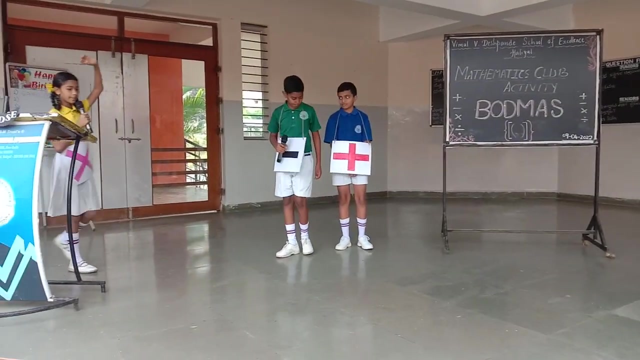 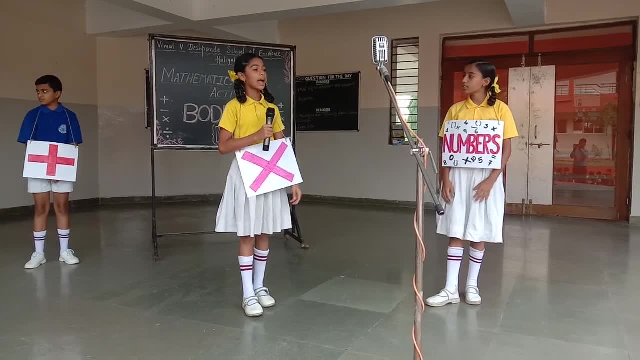 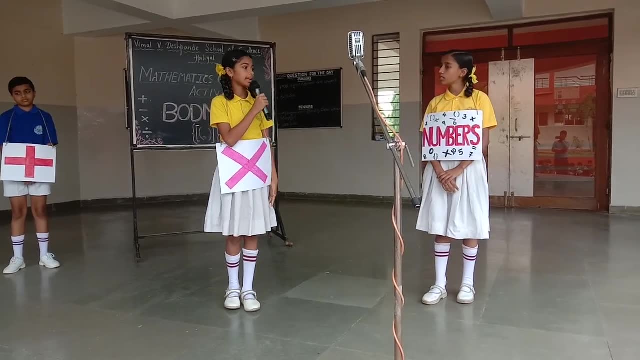 Hey, who are you? What do you mean by this? I am multiplication. I have double dots. When you want to add a number again and again, I can do it Again and again. I can make the calculation very easy. 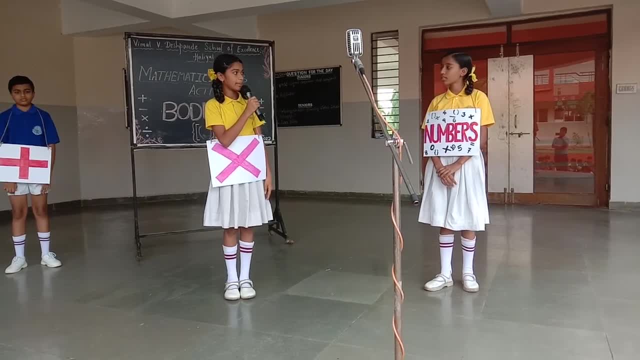 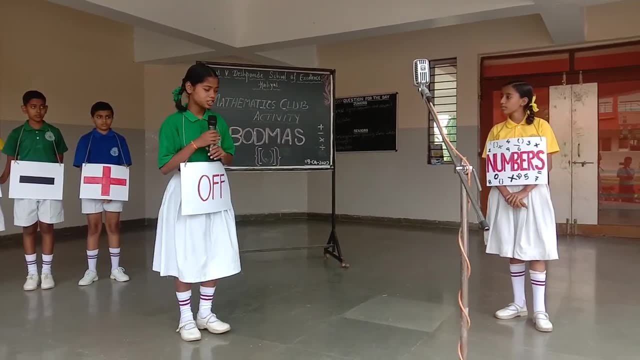 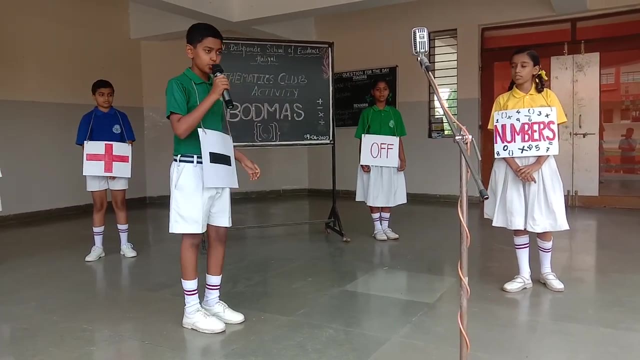 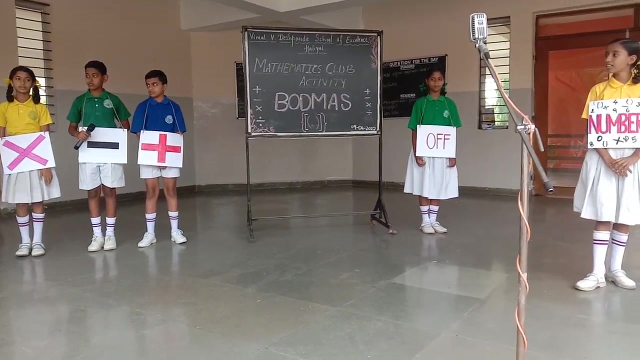 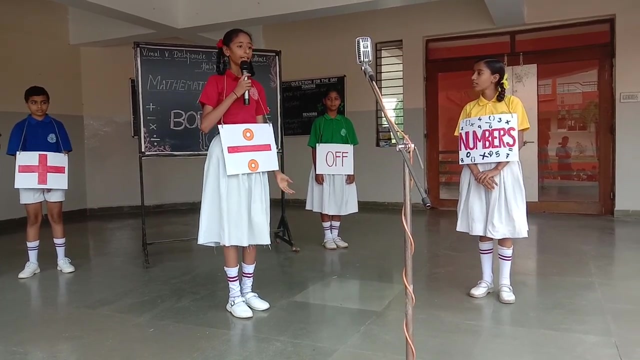 And when you call me at shortcut and tell I am in your service, I am the elder brother of multiplication, Here you go. One more operation. Do you want to meet? Yeah, I am so excited. Hi, Hello, Hi, everyone. I am division. When you want to share equally, I work into my calculation easier. 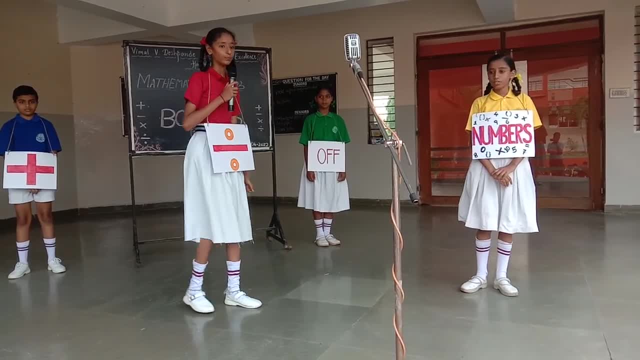 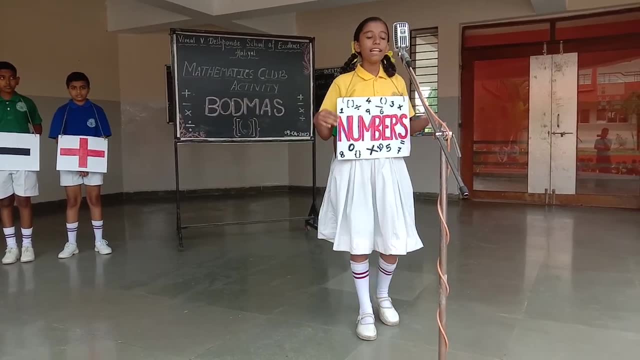 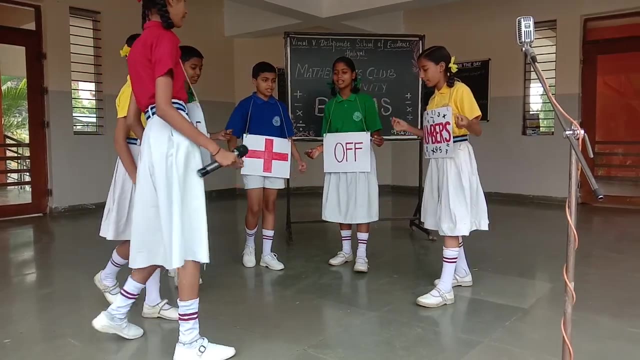